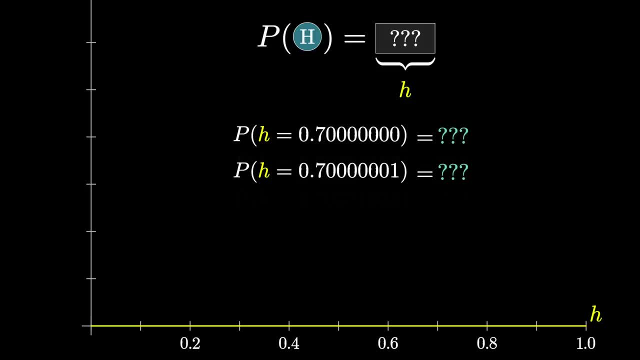 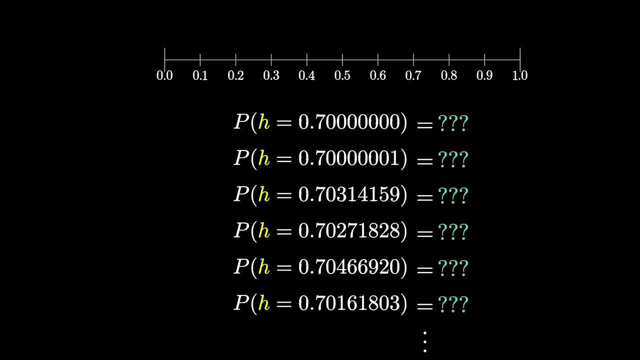 0.7,, 0, 0, 0, 0, 0,, 0, 1, or any other nearby value. well, there's going to be a strong possibility for paradox if we're not careful. It feels like no matter how small the answer to 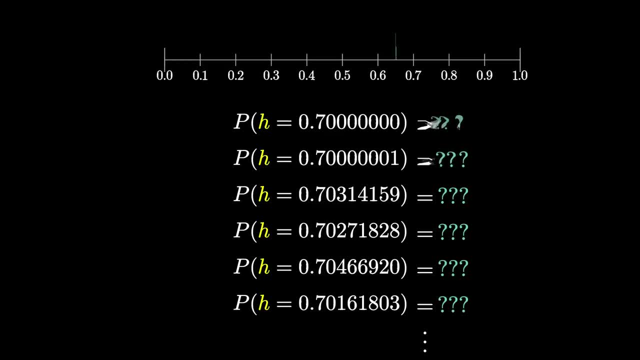 this question. it just wouldn't be small enough If every specific value within some range- all uncountably, infinitely many of them- has a non-zero probability. well, even if that probability was minuscule, adding them all up to get the total probability of any one of these. 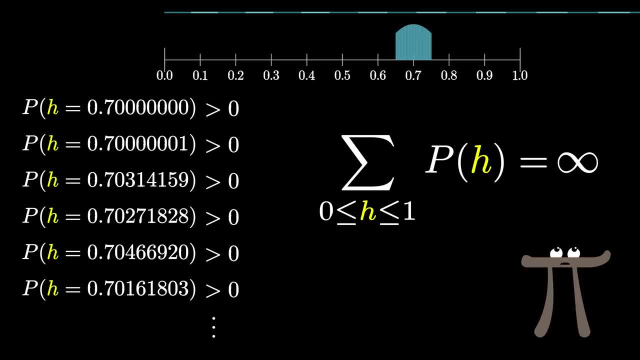 values will blow up to infinity. On the other hand, though, if all of these probabilities are 0,- aside from the fact that that now gives you no useful information about the coin- the total sum of those probabilities would be 0,, when it should be 1.. After all, this weight of the coin- h- is something, so the 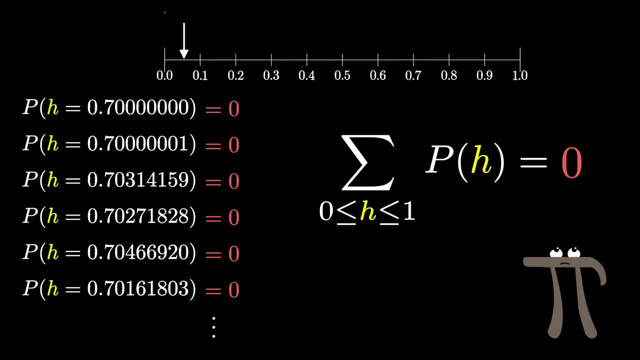 probability of it being any one of these values should add up to 1.. So, if these values can't all be non-zero and they can't all be 0, what do you do? So, if we're going to get to the point where we're going to get to the point where we're going to 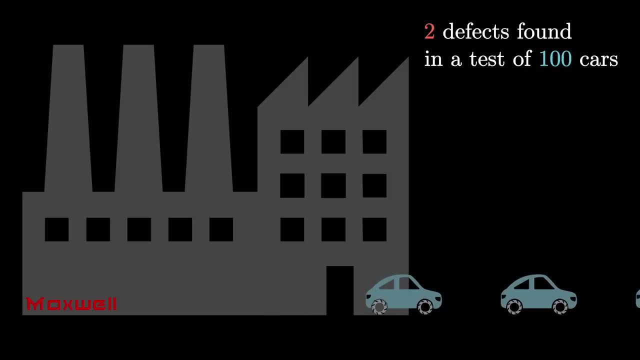 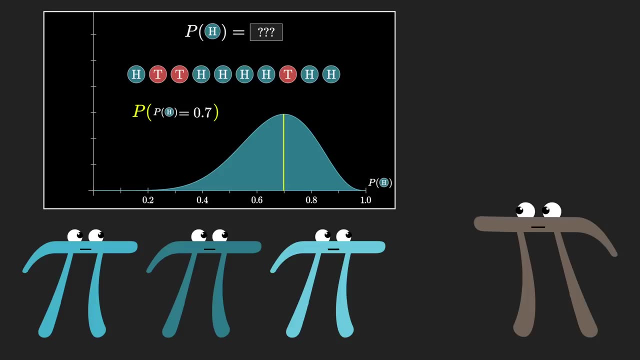 get to the point. where we're going with this, by the way, is that I'd like to talk about the very practical question of using data to create meaningful answers to these sorts of probabilities, of probabilities questions. But for this video, let's take a moment to. 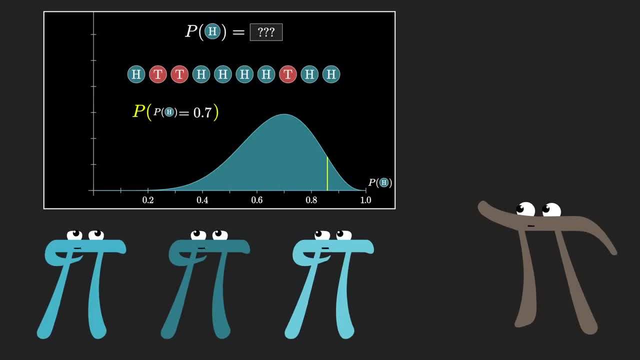 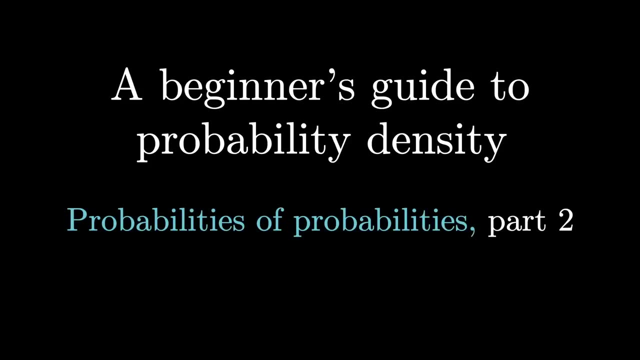 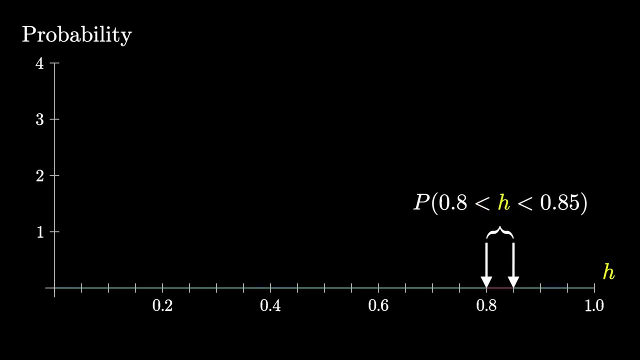 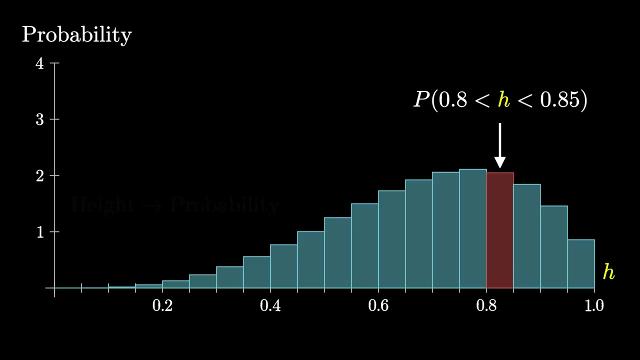 appreciate how to work with probabilities over continuous values and resolve this apparent paradox. The key is not to focus on individual values, but ranges of values. For example, we might make these buckets to represent the probability that h is between, say, 0.8 and 0.85.. Also, 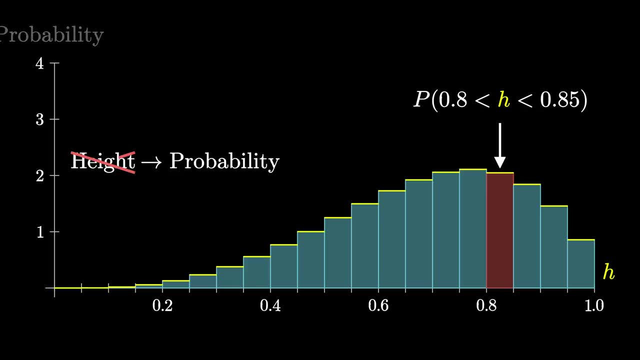 and this is more important than it might seem. rather than thinking of the height of each of these bars as representing the probability, think of the area of each one as representing that probability. Where exactly those areas come from is something that we'll answer later. 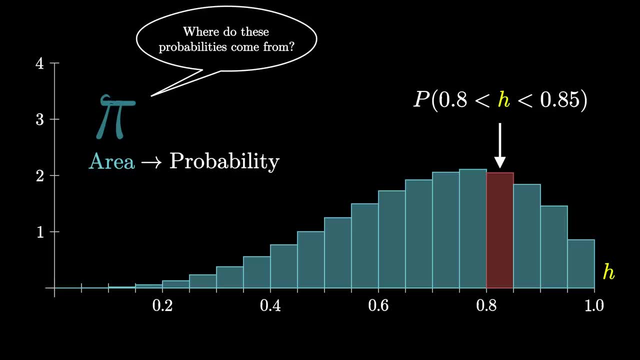 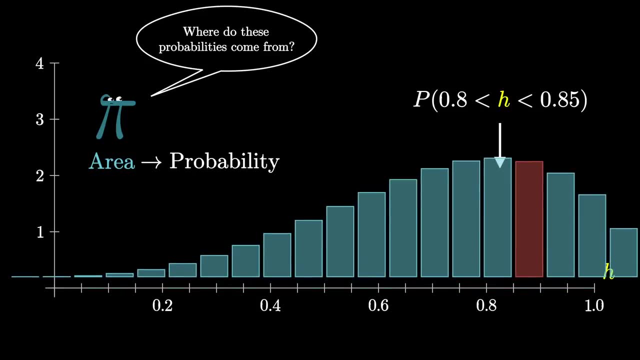 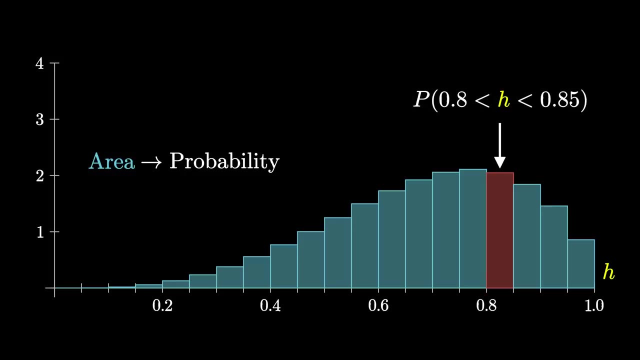 For right now just know that in principle, there's some answer to the probability of h sitting inside one of these ranges. Our task right now is to take the answers to these very coarse-grained questions and to get a more exact understanding of the distribution at the level of each individual input. The 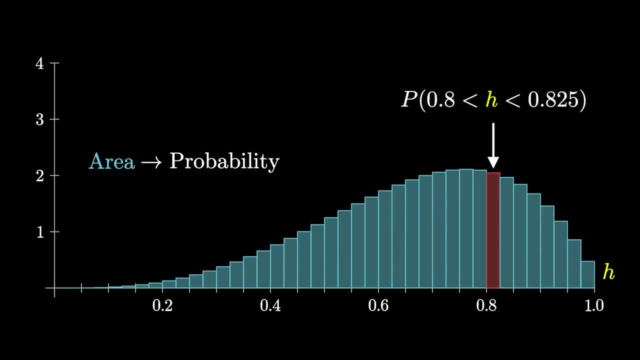 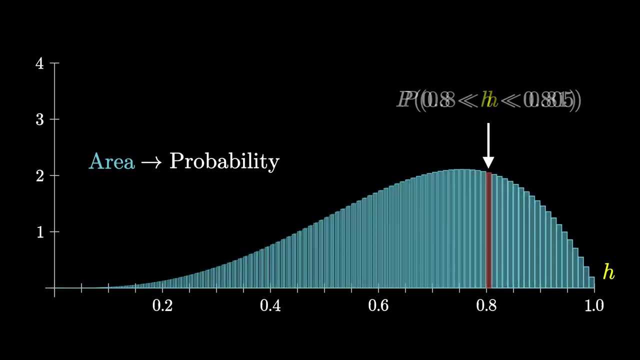 natural thing to do would be to consider finer and finer buckets, and when you do, the smaller probability of falling into any one of them is accounted for in the thinner width of each of these bars, while the heights are going to stay roughly the same. That's important. 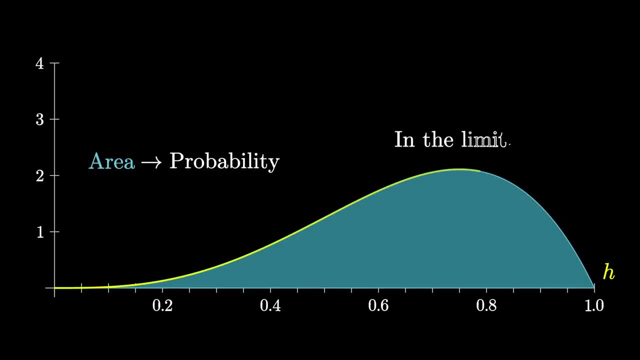 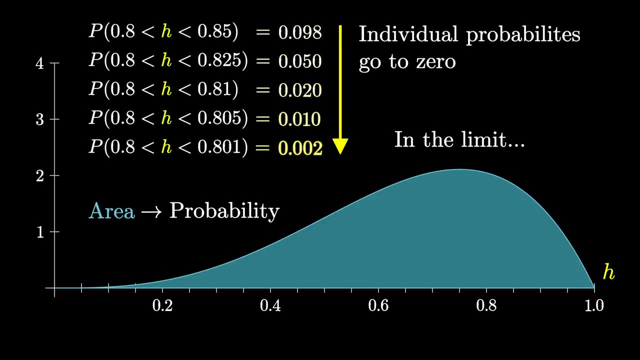 because it means that as you take this process to the limit, you approach some kind of a smooth curve. So even though all of the individual probabilities of falling into any one particular bucket will approach zero, the overall shape of the distribution is preserved, and even 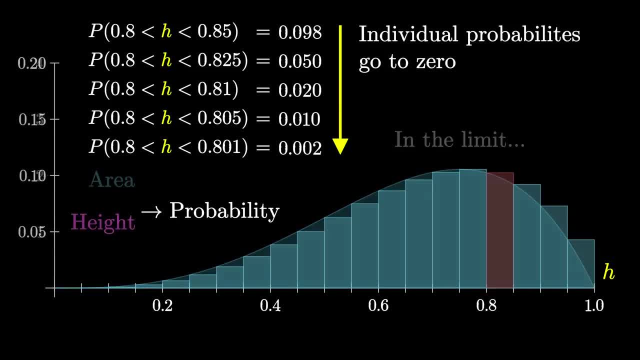 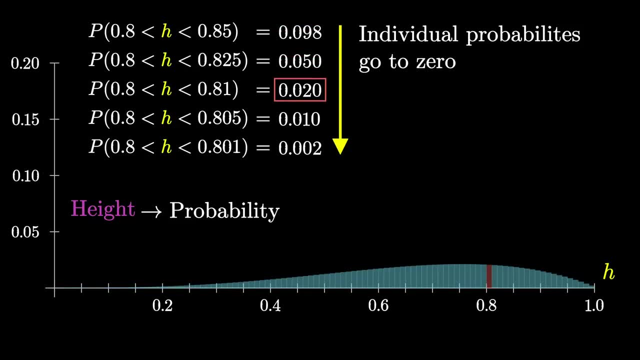 refined in this limit. If, on the other hand, we had let the heights of the bars represent probabilities, everything would have gone to zero. So in the limit we would have just had a flat line giving no information about the height of each of these bars, and we would 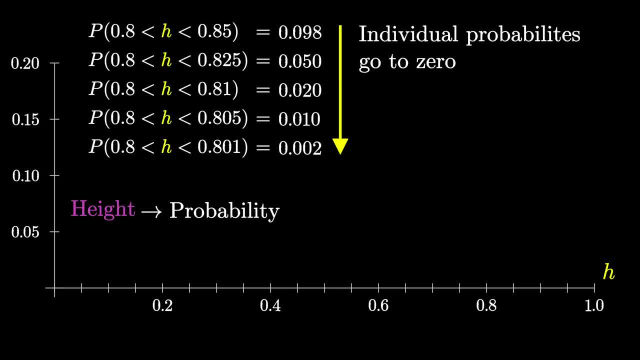 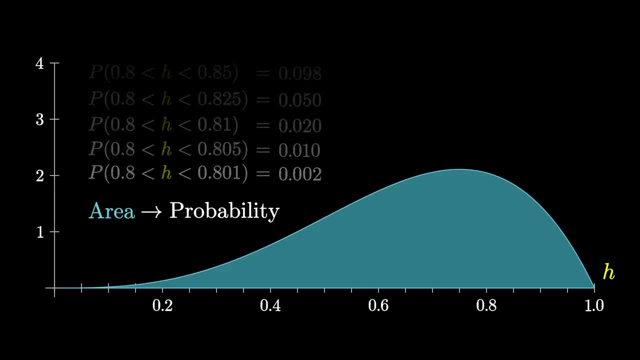 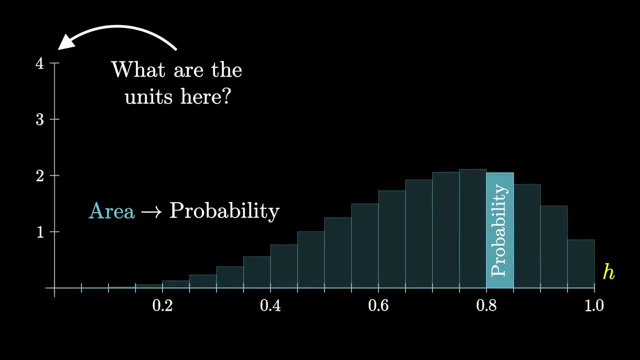 have been able to calculate the height of each of these bars. So let's think about this problem. If the Y axis no longer represents probability, then what are the units? Since probability sits in the area of these bars, or width times height, the height represents a kind of probability per unit in the X direction, what's known? 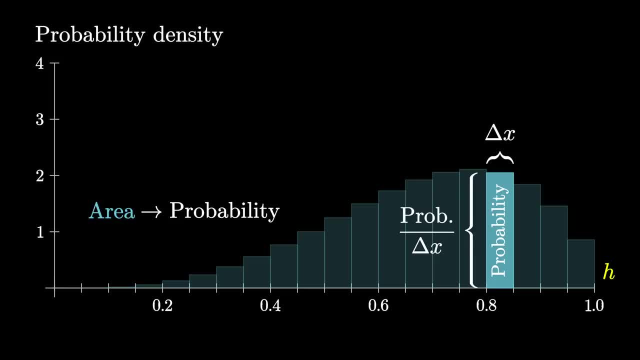 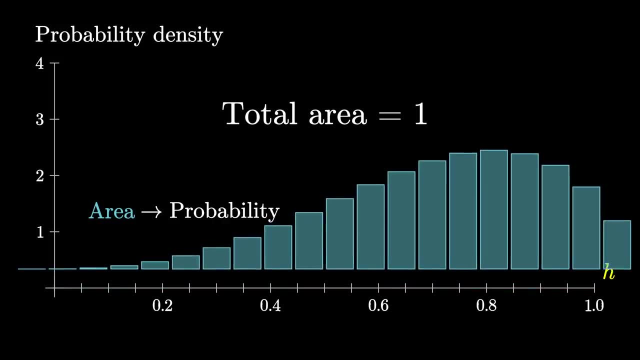 in the business as probability density. The other thing to keep in mind is that the total area of all the bars is actually the width, So what are the probability density in the bars has to equal 1 at every level of the process. That's something that has to be true for any valid probability distribution. 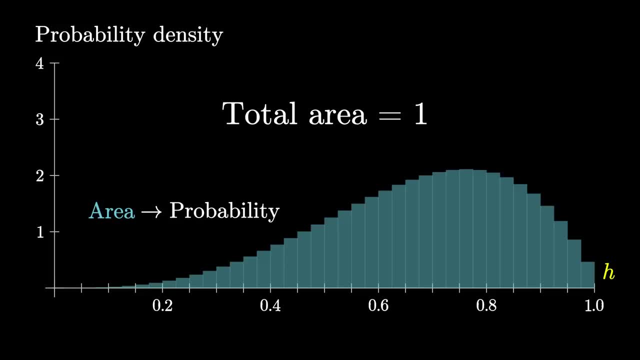 The idea of probability density is actually really clever when you step back to think about it, As you take things to the limit, even if there's all sorts of paradoxes associated with assigning a probability to each of these uncountably, infinitely many values of h between 0 and. 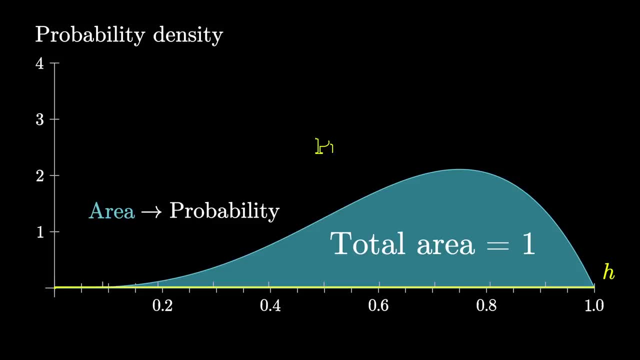 1,. there's no problem if we associate a probability density to each one of them, giving what's known as a probability density function, or PDF for short. Anytime you see a PDF in the wild, the way to interpret it is that the probability of 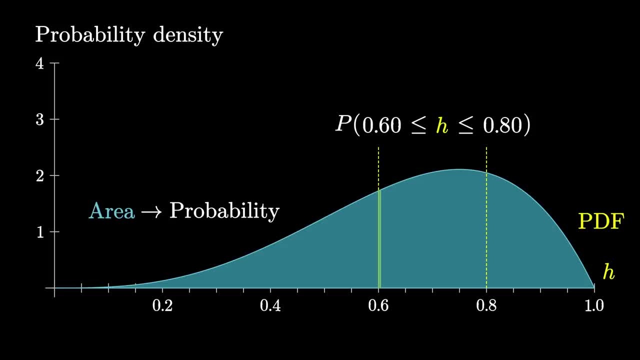 your random variable lying between two values equals the area under this curve between those values. So, for example, what's the probability of getting any one very specific number like 0.7?? Well, the area of an infinitely thin slice is 0, so it's 0.. 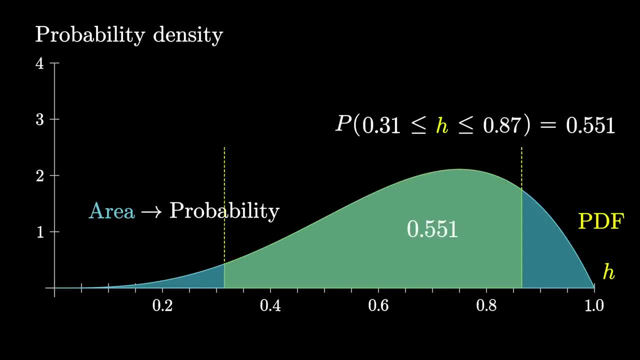 What's the probability of all of them put together? Well, the area under the full curve is 1.. You see paradox, sidestepped, And the way that it's been sidestepped is a bit subtle. In normal finite settings like rolling a die or drawing a card. the probability that 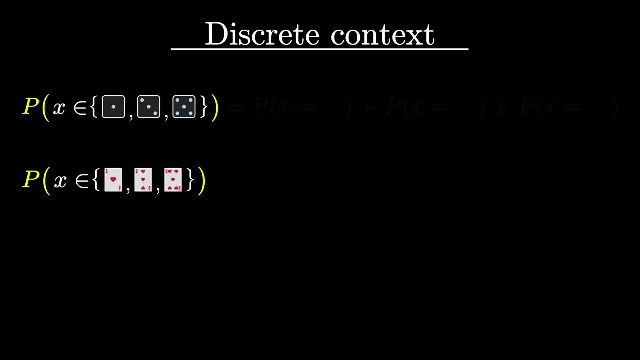 a random value falls into a given collection of possibilities is simply the sum of the probabilities of being any one of them. This feels very intuitive. it's even true in a countably infinite context. But to deal with the continuum, the rules themselves have shifted. 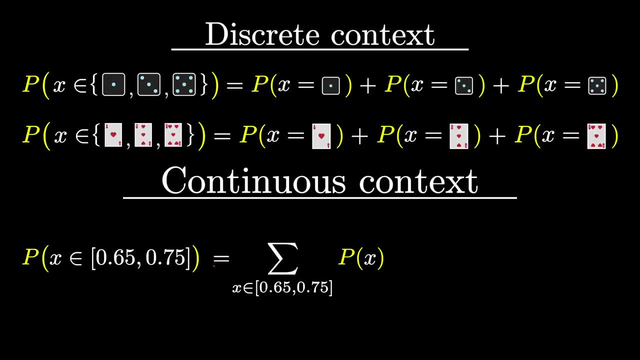 The probability of falling into a range of values is no longer the sum of the probabilities of each individual value. Instead, probabilities associated with ranges are the fundamental primitive objects And the only sense in which it's meaningful to talk about an individual value here is 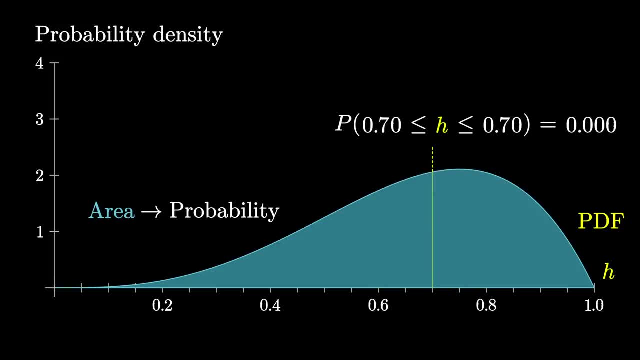 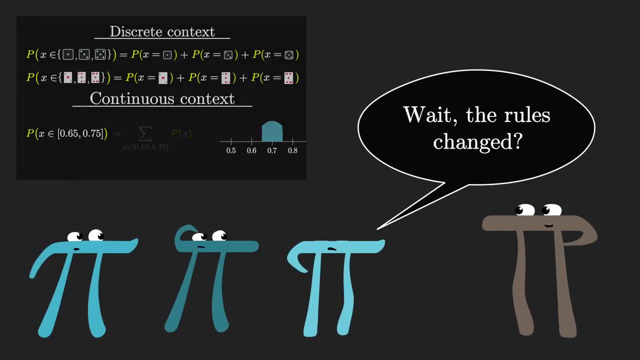 to think of it as a range of width 0.. If the idea of the rules changing between a finite setting and a continuous one feels unsettling, well, you'll be happy to know that mathematicians are way ahead of you. There's a field of math called measure theory, which helps to unite these two settings, and 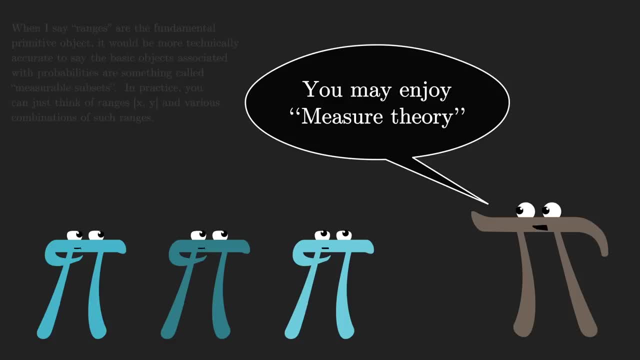 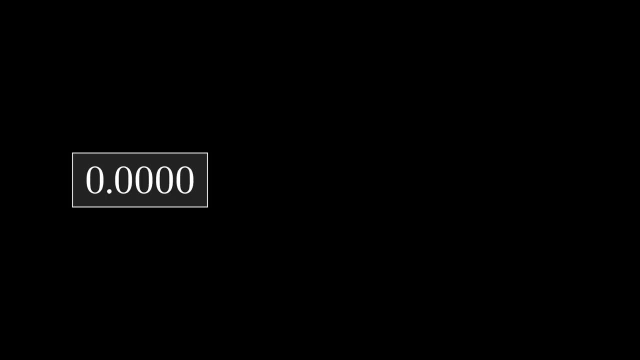 make rigorous the idea of associating numbers, like probabilities, to various subsets of all possibilities in a way that combines and distributes nicely. For example, let's say you're in a setting where you have a random number that equals 0 with 50% probability, and the rest of the time it's some positive number. according, 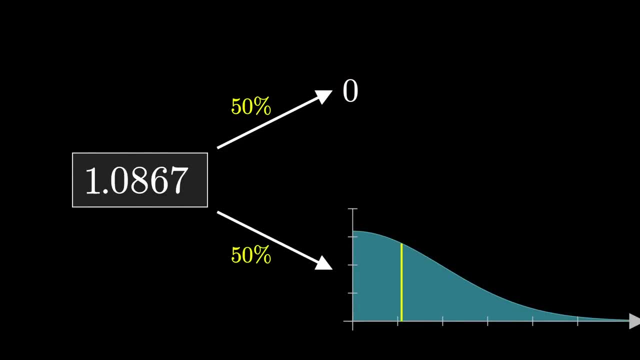 to a distribution that looks like half of a bell curve. This is an awkward middle ground between a finite context where a single number is a single value with a non-zero probability, and a continuous one where probabilities are found according to areas under the appropriate density function. 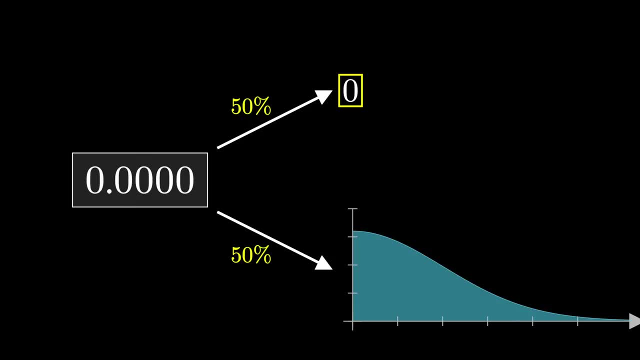 This is the sort of thing that measure theory handles very smoothly. I mention this mainly for the especially curious viewer, and you can find more reading material in the description. It's a pretty common rule of thumb that if you find yourself using a sum in a discrete 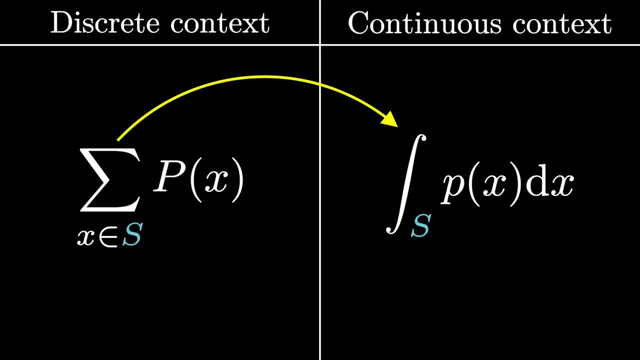 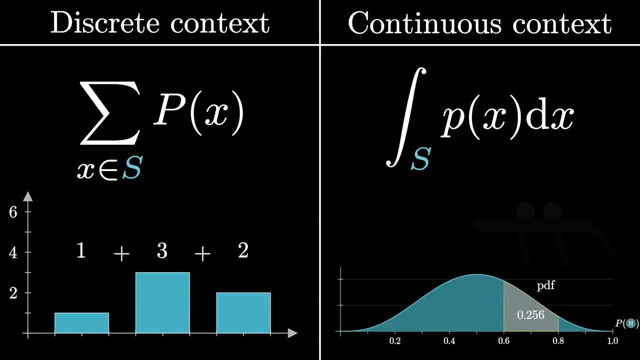 context, then use an integral in the continuous context, which is the tool from calculus that we use to find areas under curves. In fact, you could argue this video would be way shorter if I just said that at the front and called it good. 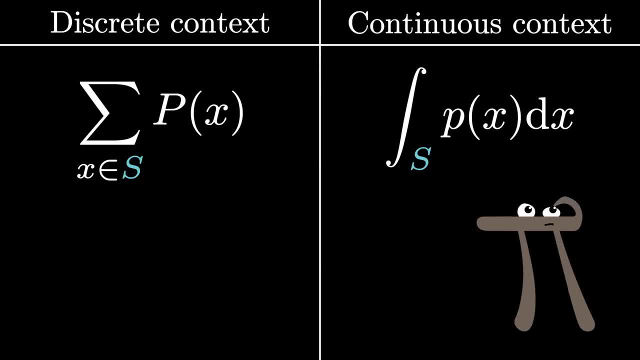 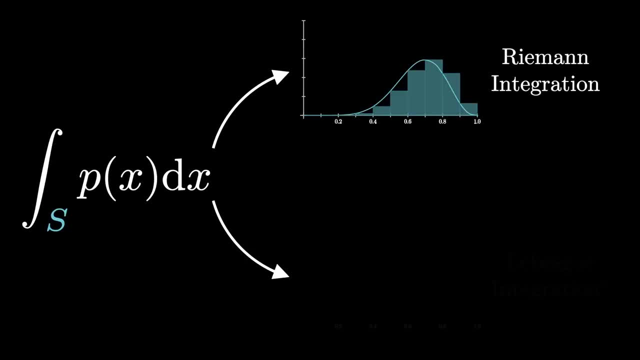 For my part, though, I always found it a little unsatisfying to do this blindly, without thinking through what it really means. And, in fact, if you really dig into the theoretical underpinnings of integrals, what you'd find is that, in addition to the way that it's defined in a typical intro calculus class, 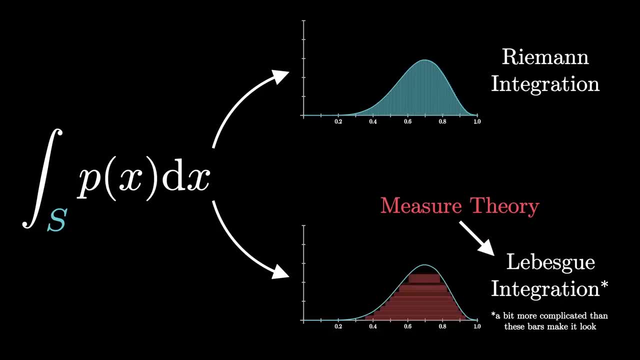 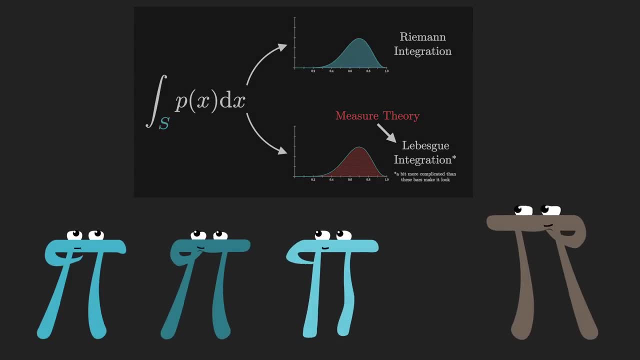 there is a separate, more powerful definition that's based on measure theory, this formal foundation of probability. If I look back to when I first learned probability, I definitely remember grappling with this weird idea that in continuous settings, like random variables that are real numbers or 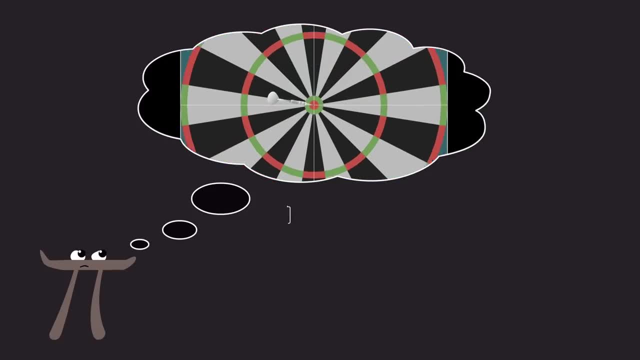 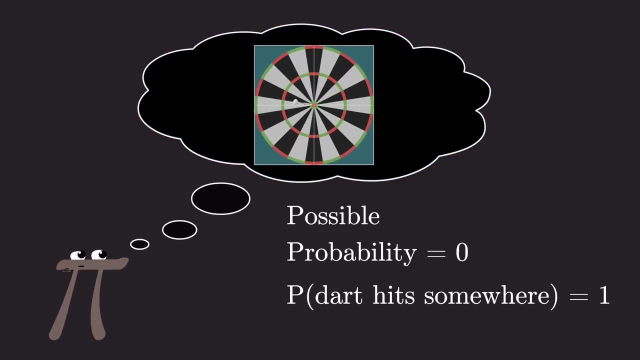 throwing a dart at a dartboard. you have a bunch of outcomes that are possible, and yet each one has a probability of zero, and somehow altogether they have a probability of one. One step of coming to terms with this is to realize that possibility is better tied to. 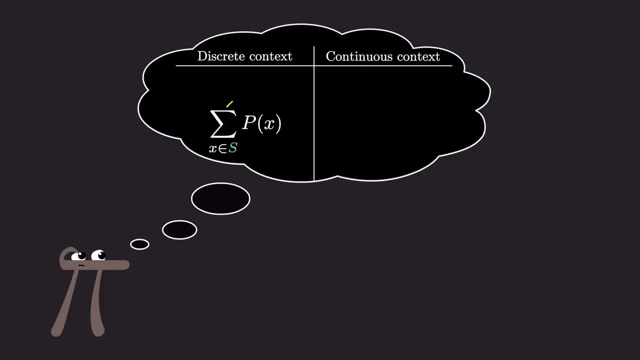 probability density than probability. However, Popping out sums of one for integrals of the others never quite scratched the itch for me. I remember that it only really clicked when I realized that the rules for combining probabilities of different sets were not quite what I thought they were, and there was simply a different. 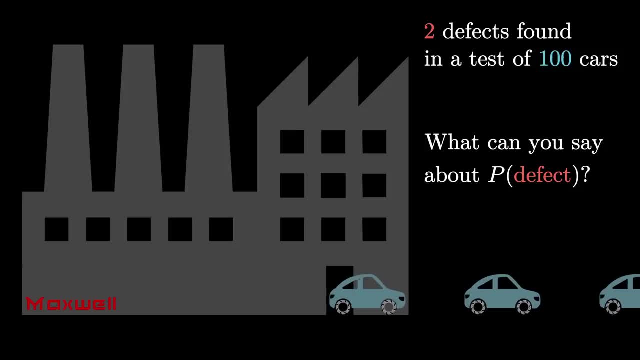 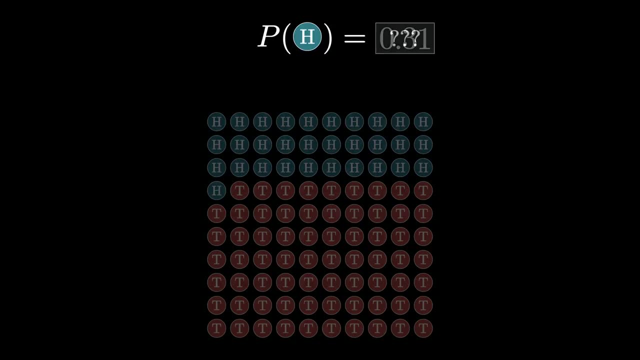 axiom system underlying it all. But anyway, steering away from the theory somewhere back in the loose direction of application, look back to our original question about the coin with an unknown weight. What we've learned here is that the right question to ask is: what's the probability? 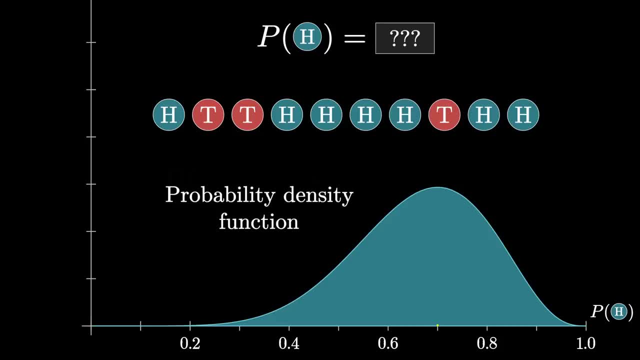 density function. What's the probability density function that describes this value h after seeing the outcomes of a few tosses? If you can find that pdf, you can use it to answer questions like: what's the probability that the true probability of flipping heads falls between 0.6 and 0.8?? 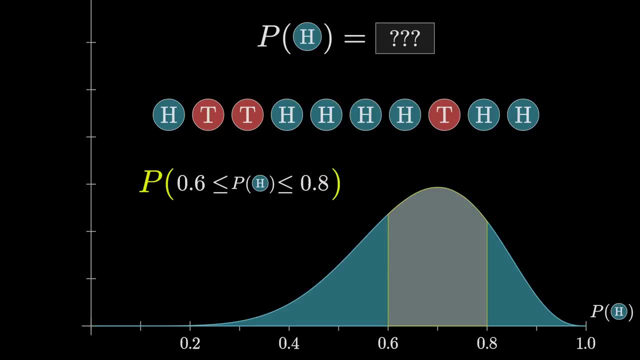 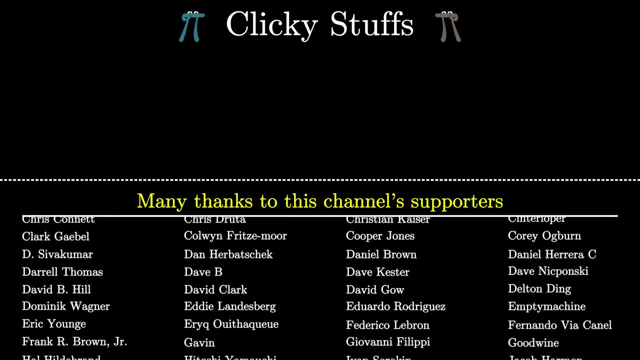 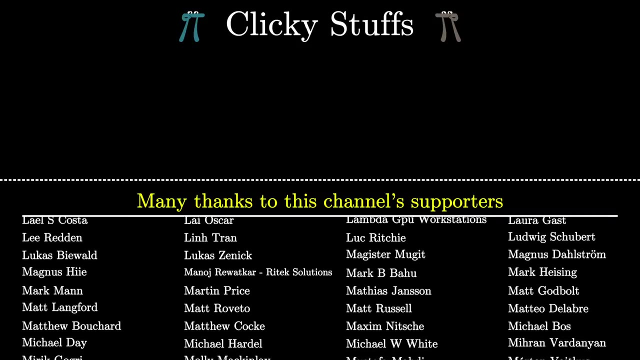 To find that pdf. join me in the next part. Thanks for watching. I'll see you next time. Bye, Bye, Bye, Bye.